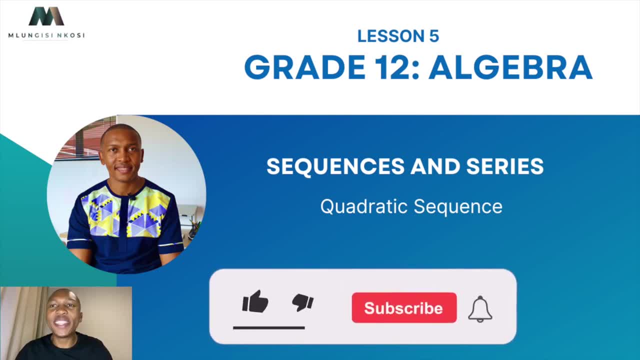 And for those of you who are new to the channel, please just welcome And please consider subscribing to our channel And please be part of the family. Okay, And please don't forget to hit that notification bell. And for those of you who may need extra assistance, of course we are available And our email address is info at mlumisengosicoza. 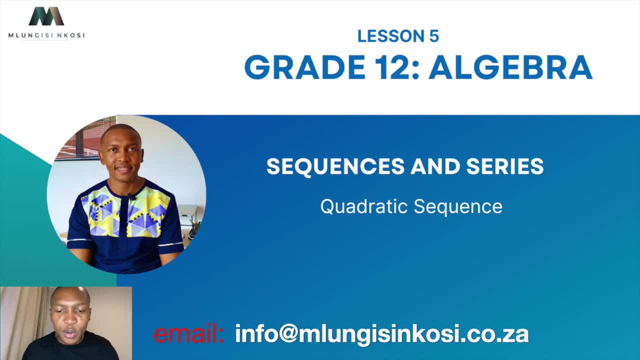 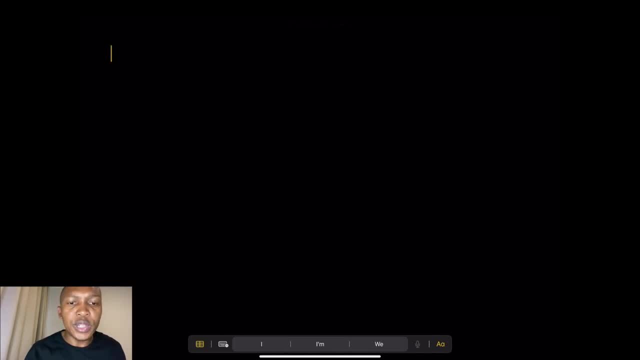 All right, so let's get into our lesson quickly. So today we're looking at the quadratic sequence. So one of the things that we just need to just remember is that when we think of a quadratic expression, okay, so we say the general term of a quadratic sequence, this is going to be: Tn is equals to An squared plus Bn plus C. All right, so this is what we call the general term of a quadratic sequence. 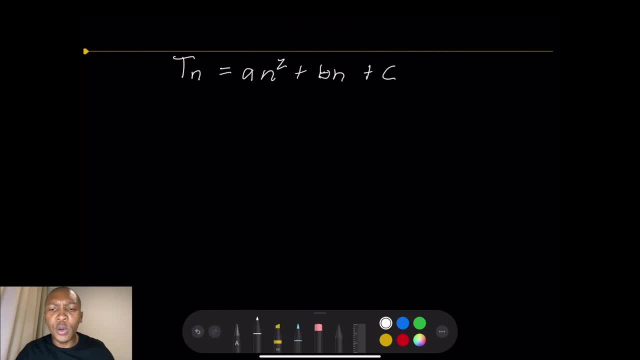 Now, as you would know. so, in order for us to express that general term, what we do need is to find out what the value of A is and what the value of B is, as well as the value of C. Okay, so we're going to look at just exactly how we are going to do that Now. I'm going to show you two methods. Okay, I want us to take a quick example. All right, so let's take a. you know a sequence. In fact, I just had it in front of me. 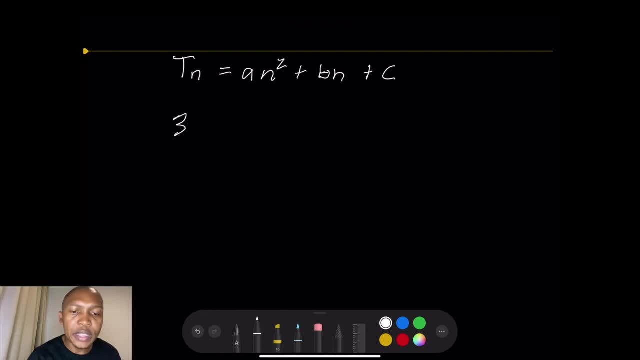 Just now. Okay, so suppose we've got three, we've got nine, we've got 17, and 27.. Okay, of course you can continue that, that that probably the next one would be 38, and so on and so forth. Now there are two things that you, that I want us, to look at. So, first of all, what do we, how do we identify a quadratic sequence? So what makes a quadratic sequence? 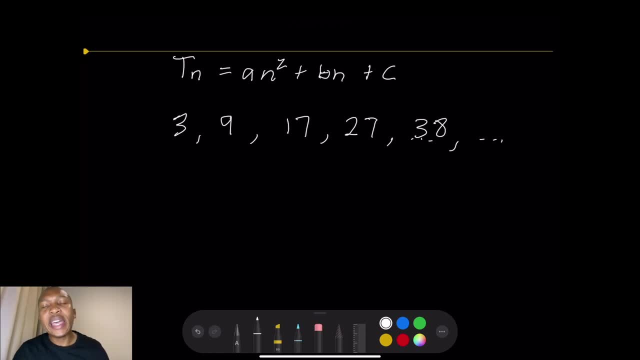 A quadratic sequence, Okay. so you'll see that there is no constant difference, there's no common difference between the terms. All right, so this is term one, okay, and term two. And you realize, if I take term one minus term two, as we would for an arithmetic sequence, So if we say term one minus term two, this would give us six. If I say term two, term three, divided by two, 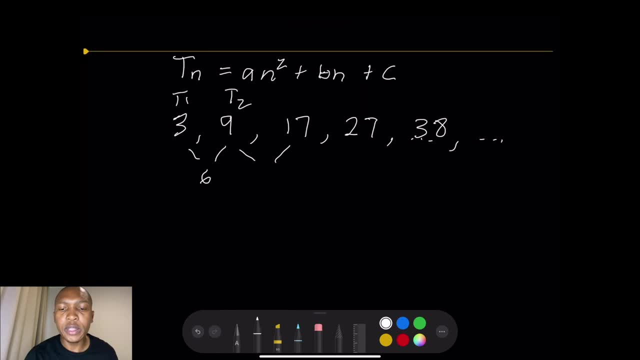 I mean minus term three, rather minus term two. this would give me, you know, that would give me eight, Okay. and if I say, you know, term four minus term three, that would give me a 10, for instance, And of course you'd see that as it continues. So sorry, I think that was incorrect. 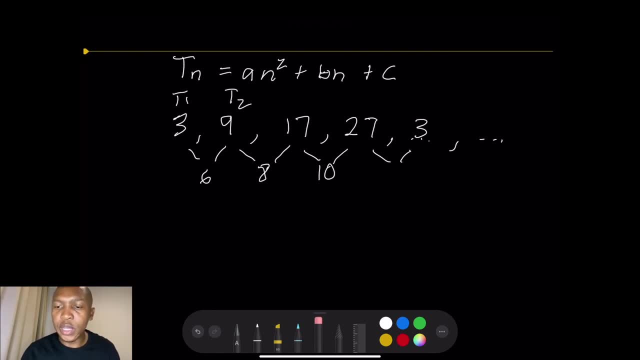 There. Yeah, so that should have actually been a different value, Right? so, and you'll continue so on and so forth. Now you'll see, there is no common difference between the terms, right? However, with a quadratic sequence, there is a common, a constant, second common difference. Now I want you to look at this. So this 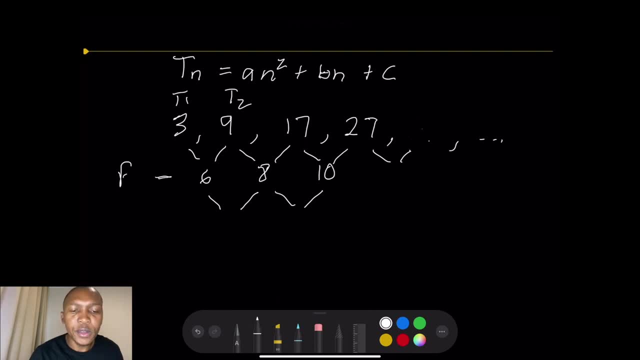 would be the first difference here. Okay, so this would be: look at me writing fist instead. Okay, so this would be the first difference. And then now let's take the second difference. It means that we are taking the difference of the difference. Okay, so we're simply saying eight minus six, that would give us two, And, of course, 10 minus eight, that would also give us two. So 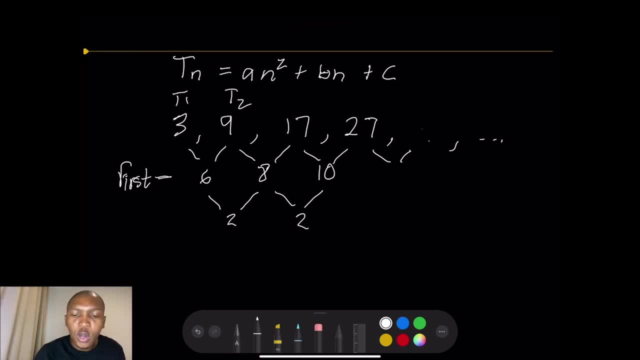 when you look at it, there is now a common difference, but it's only the second difference that is common. So in this case, we've got a common second difference. Now there's a way in which we can do this, And I want us to just explore a couple of ways. how are we going to get the values of a, b and c with this? Now, of course, I you know there's a. there could be a. 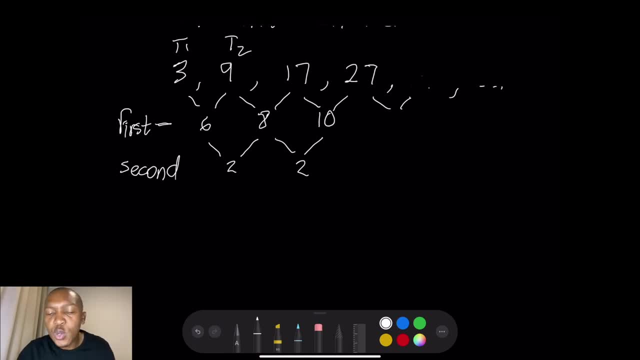 difficult method in which you can do this. Let me just show you quickly what you could do. So what you could do in the first instance is just to simply say: well, look, I will substitute what I know. Of course I've got term one, term two and term three. So what you could do is just simply say: well, what is my term? Of course you've got the general, you know sequence, So you can say: 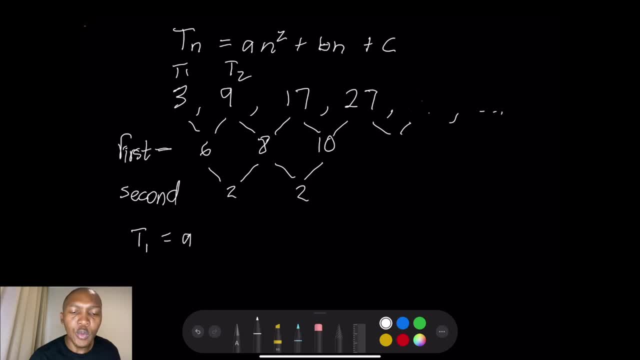 well for term one. I don't know what value of a is, but I know that this is going to be one squared plus b times one plus c. Okay, so you end up with a plus b plus c. Okay, just keep in mind this must might come in handy earlier on. I mean later on. So then this would be my first equation, Of course. then you can say: well for term. 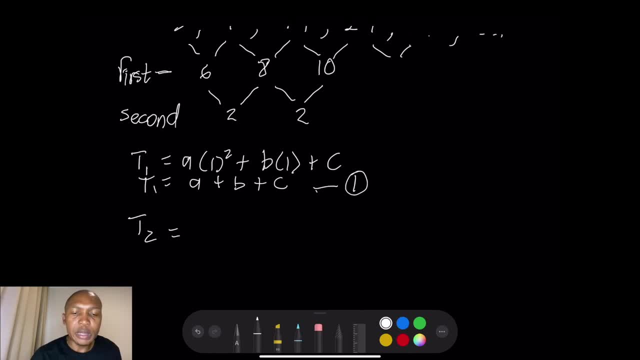 two. all I just simply do is just substitute two for the value of n, So I've got a times two squared plus b, times two plus c again. Okay, and this would be equation two In fact. let's do this. So this would be for a plus two, b plus c, And this would be our. 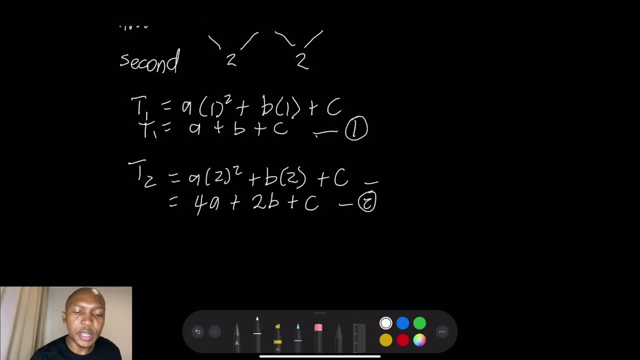 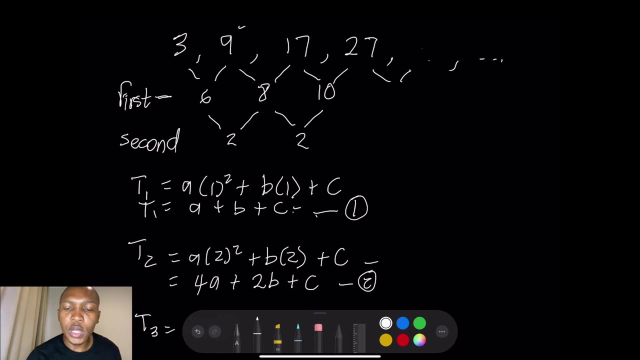 equation two. And of course you do the same for term three. you'd say term three. this is a three squared plus b. Sorry, in fact, I keep forgetting to just substitute what we know. We know the value of each term. So a plus b plus c- sorry, is equal to three in this case. Okay, Sorry, I'm just going to add that. 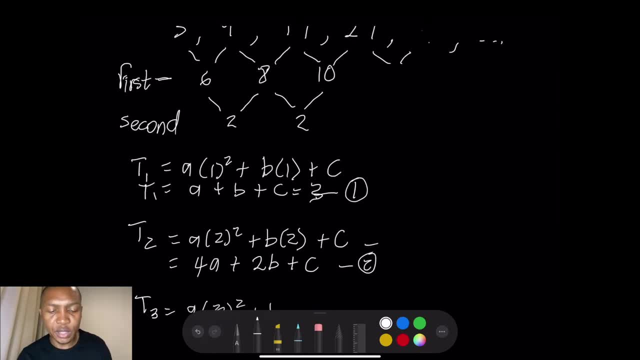 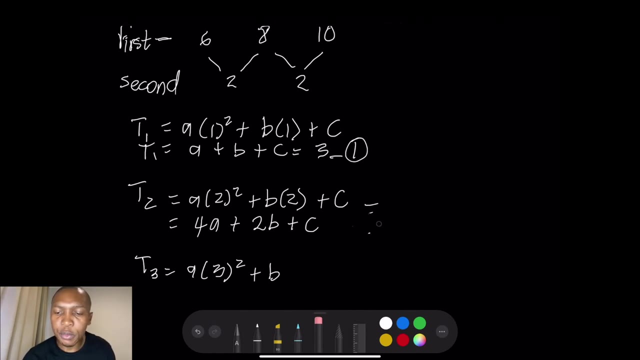 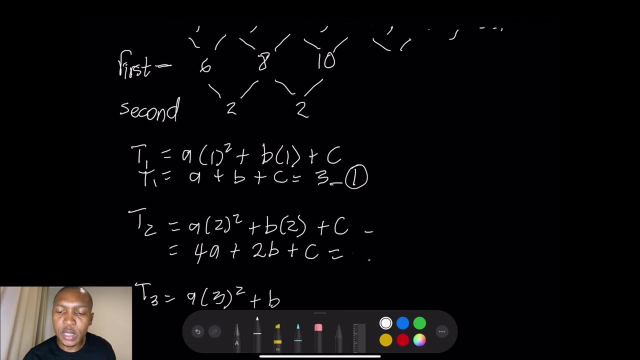 Hope it's not too bad. Okay, maybe I just need to. Yeah, let's just remove that. Okay, so this is going to be three, And this is our equation one, And then for equation two, of course, just removing that again, Our our term two is nine. Okay, so all of that is equal to nine, And that would be our equation two. 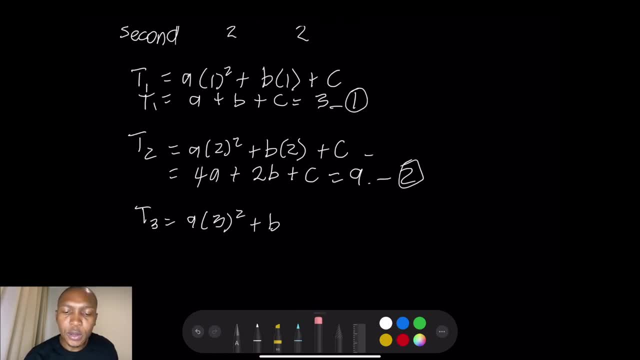 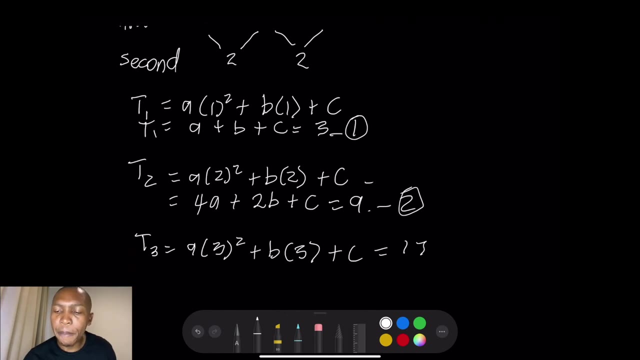 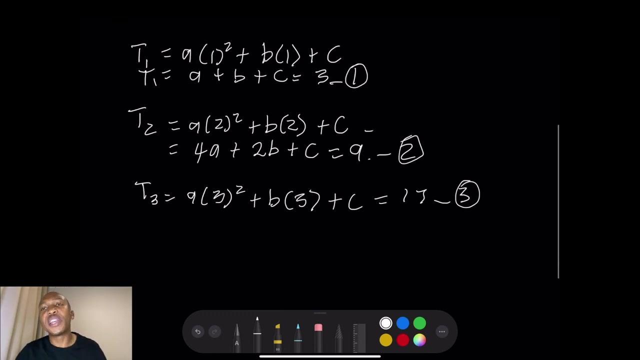 And, of course, for the third term. okay, so this is multiplied by three, plus c again, and which is equal to our third term, in that case was 17.. Okay, And this would be equation three. Now, of course, what are you going to do? you're going to try and solve simultaneously. I'm not about to do that. Okay, you can see how. 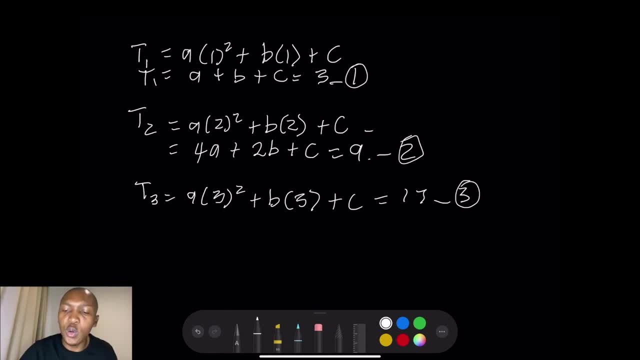 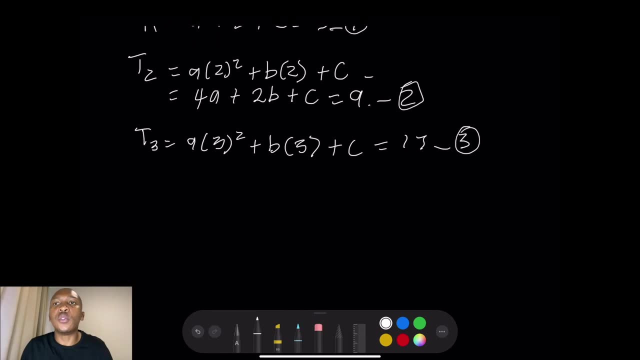 that would be quite a tedious exercise, But what I want to quickly show you is how to do that. you know, in sort of an easier way, but it just requires you to commit certain things to memory. Okay Right, How would we do this in you know, in somewhat of an easier way to follow? Okay right, You can try and solve that simultaneously. you know, get to the answer, But let me show you this particular method. 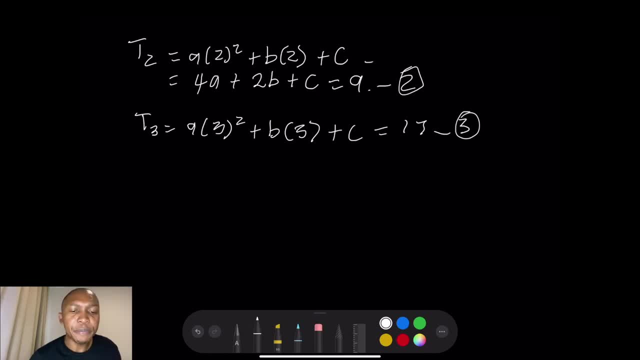 So what we would need to keep in mind. okay, as I did say to you, I want you to keep certain things in mind. So 2a will always be the second difference. Okay Right, I'm just going to call it s. So 2a will always be equal to the second difference. 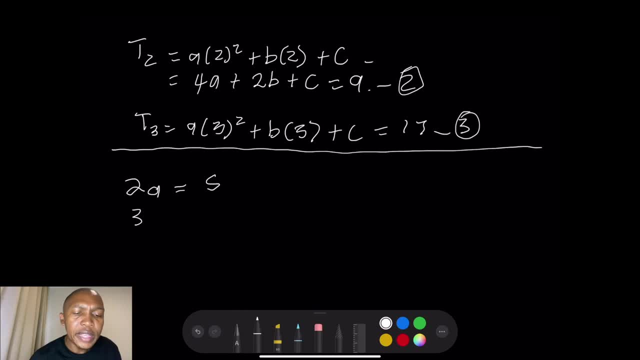 And then 3a plus b- Okay, Is equal to our first difference. Okay, So, first difference. I don't know why I wrote it out fully there. Okay, maybe let me write it. second difference: Okay, All right, And then, when it comes to finding out the value of c, all you simply do is just go back to that equation that we made. 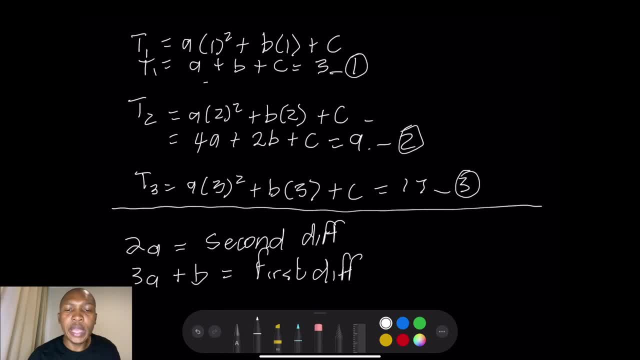 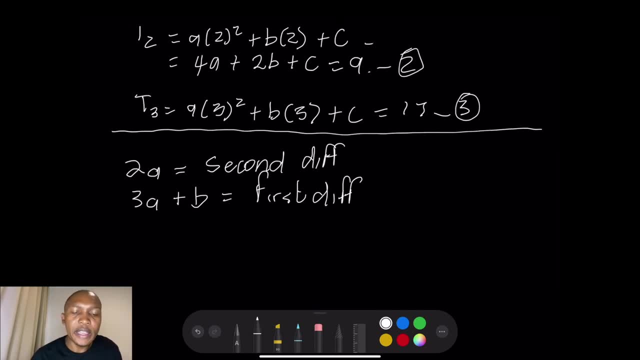 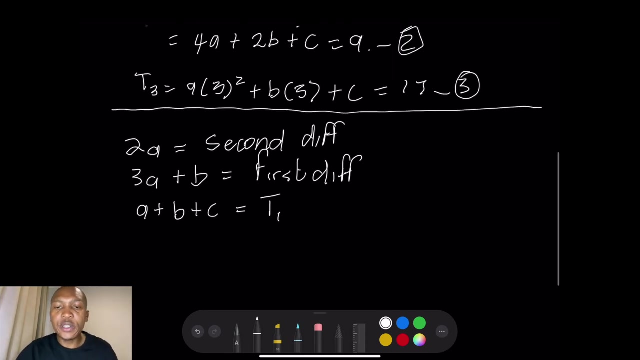 There for term one. Okay, we know that term a plus b plus c would be equal to three there. So we can just simply say: to get the value of c, all I simply do is say a plus b plus c is equal to the first term. Okay, Right Now, what I want us to do quickly is let's try to solve, you know, for this particular quadratic sequence. 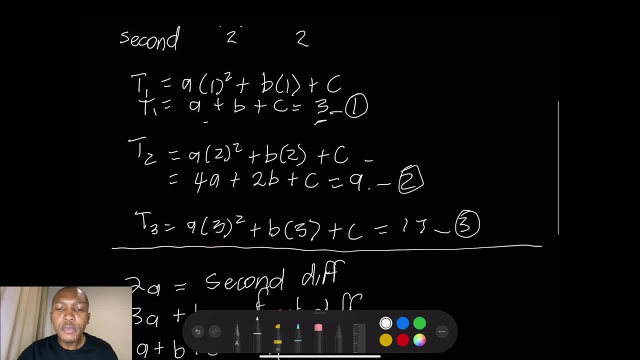 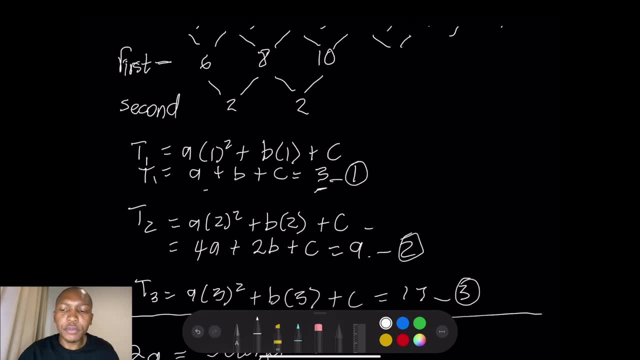 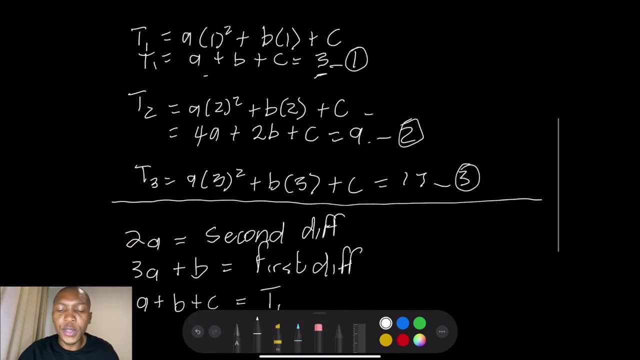 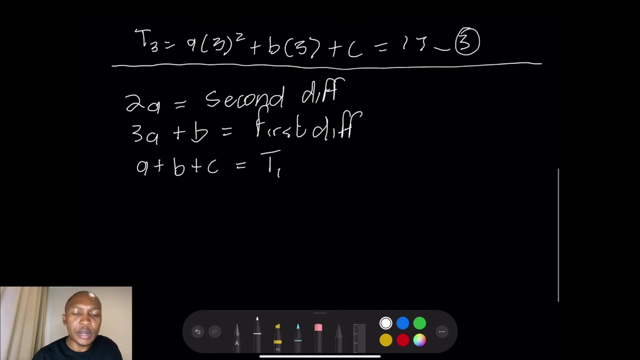 To what are the values of a, b and c? All right, Just keeping in mind. All right, We already found the first difference. Okay, So the value of the first, or the first term of the first difference, I should have said for the first one. Okay, So this would be the first term of the first difference. So in this case, I'm going to say: right, let's find out what the value of a is. 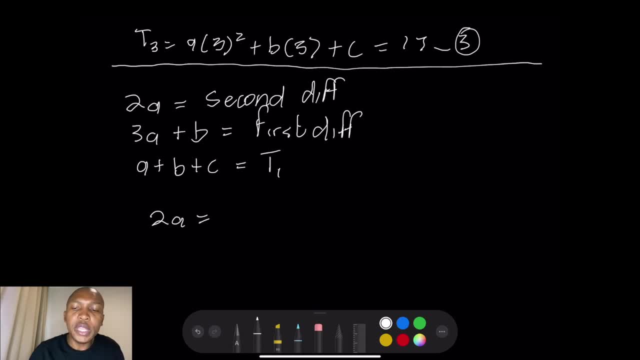 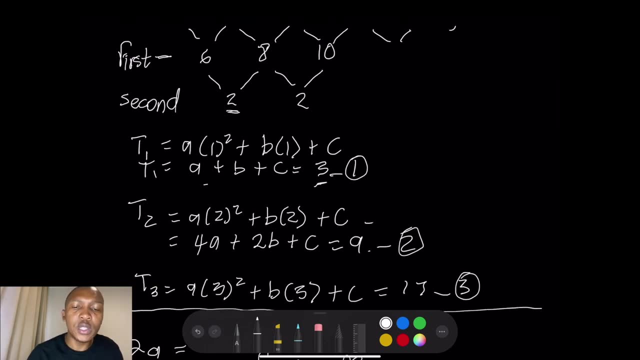 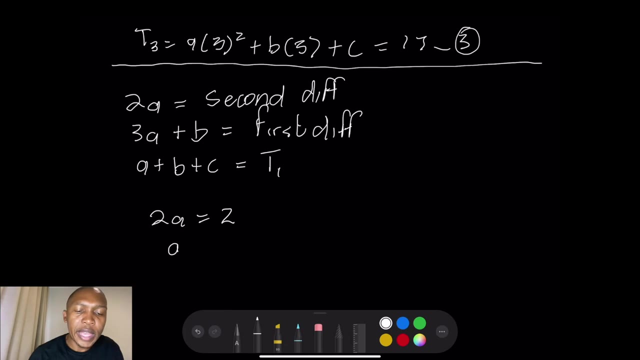 So we know that 2a Would be equal to what was our first, our second difference. Our second difference in this case was two. So 2a is equal to two. So then, solving for a, then it means that a is equal to one. Okay, Right. And then then we go to our second equation. We know that 3a plus b is equal to. 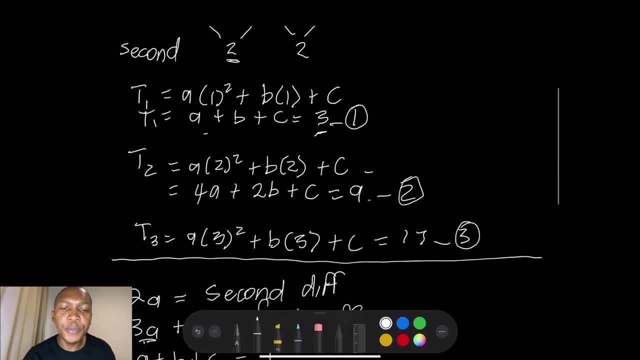 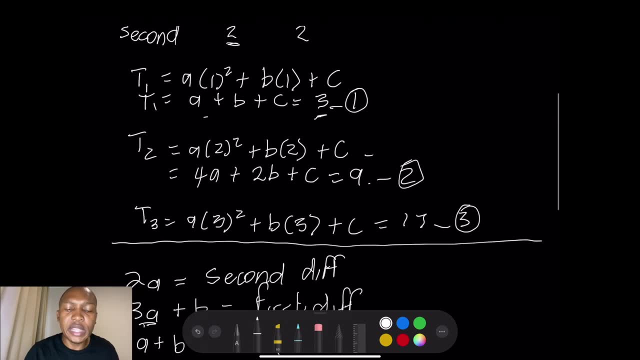 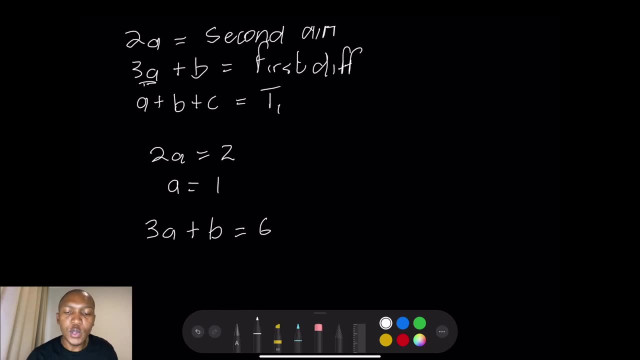 Now, please, I want you to note Where do we get the value. That would be the first term of the first difference. So it means that 3a plus b would be equal to six in our case. Okay, So that would be equal to six, but we already have the value of a. So it means that three multiplied by one- we can substitute for a there- plus b is equal to six. 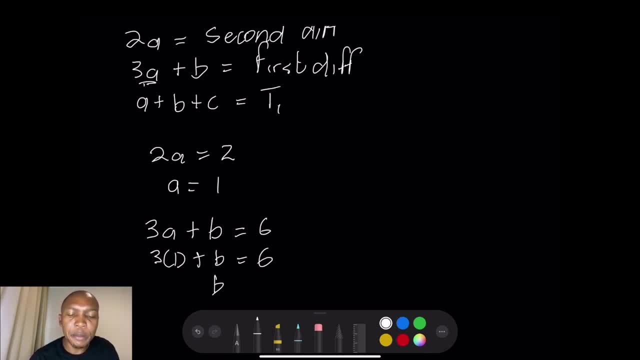 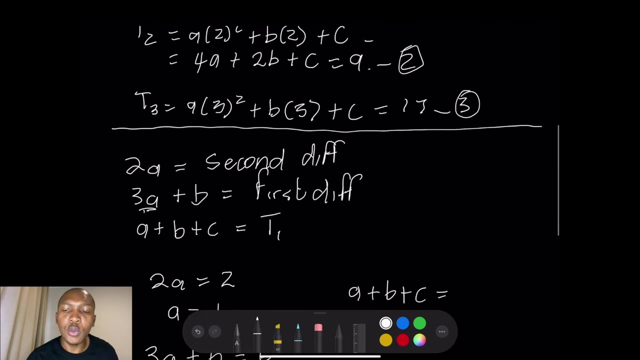 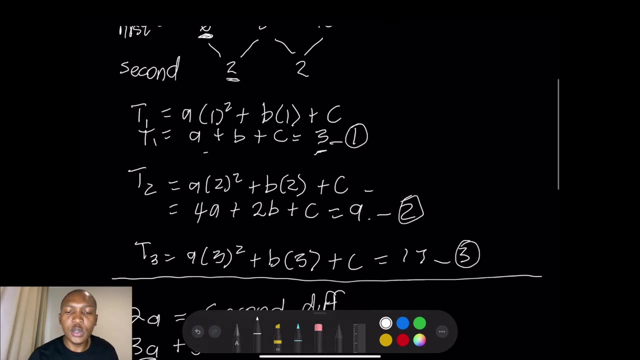 And, of course, if you solve three times, one is three, So that the b value is equal to. so that six minus three, that would be equal to three. And finally, what would be our value for c? So we know that a plus b plus c would be equal to the first term. Now note what is our first term of the sequence. Said our first term was three. So in this case it's actually that equation over there. 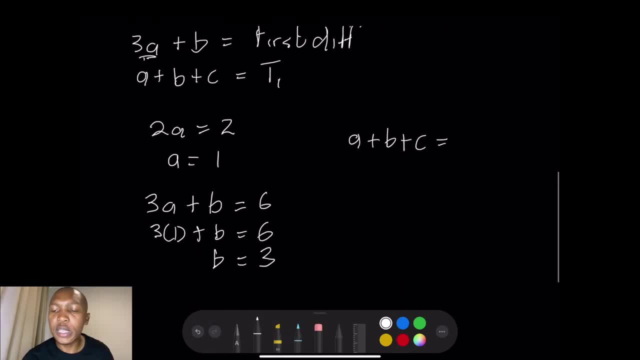 Okay, So a plus b plus c is equal to three. Okay, And so all that, you simply do remember. we already know the value of a. a, we said it's one, And we know the value of b to be three, And we are looking for the value of c In this case, which is, which is all, which all of them are equal to three, And then, in this case, to get the value of c, I'll say three. 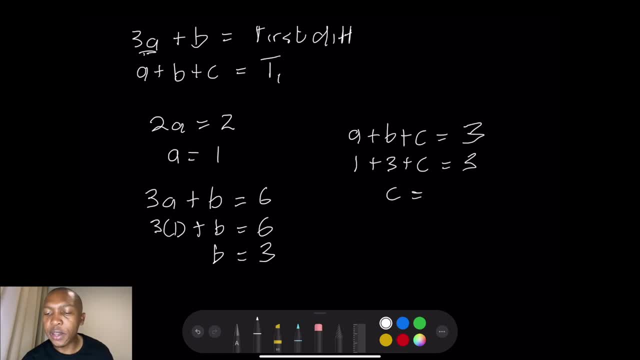 Okay, So that's our c value. So it means to get the general term of the sequence. Now, remember, now I've got the value of a, I've got the value of b and I've got the value of c. So t n- please note- is equal to- yeah, I'm trying to erase that- is equal to. my value of a is one. 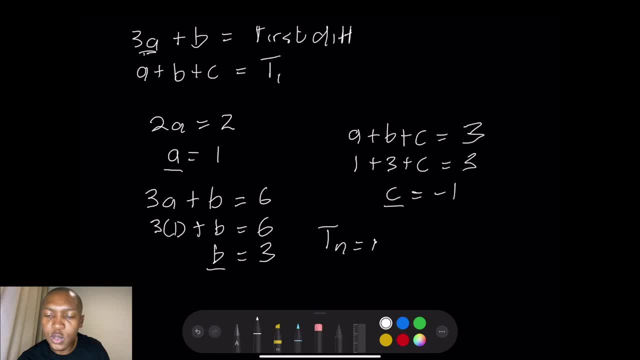 Okay, So that's going to be equal to c. Okay, And so that's the트 value to be one n squared. so this is going to be n squared plus. in this case, our b is positive. so this is plus three n and minus one. so that is how we will get the general term of our sequence, and 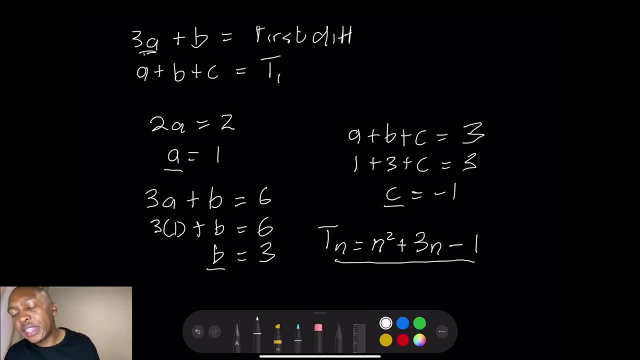 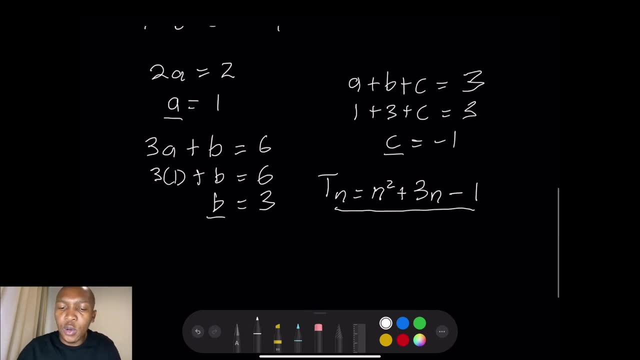 of course, from this: if they say, find the tenth term, all you simply do is just substitute ten there. okay, and i hope that was, um, uh, you know, very easy to follow and very easy to understand. all you need to do is just remember. you know, you're just committing to memory these three things. 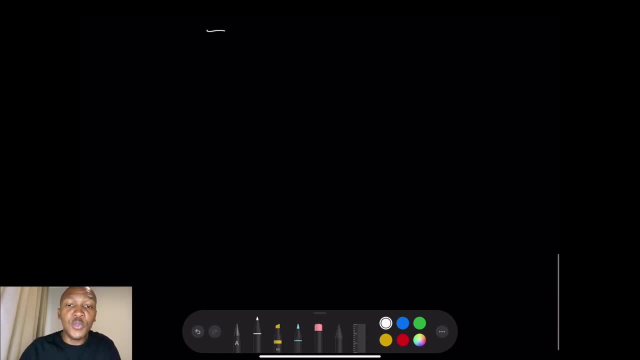 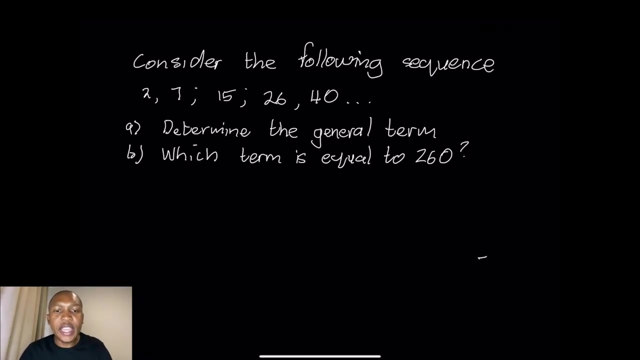 and, uh, you know, you, you, you go for it. okay, right, uh, what i would like us to do is maybe just take another example. okay, um, you know, uh, maybe the one that looks a little bit different, okay, and let's do exactly that, all right, uh. so for our second example, they say: consider the following: 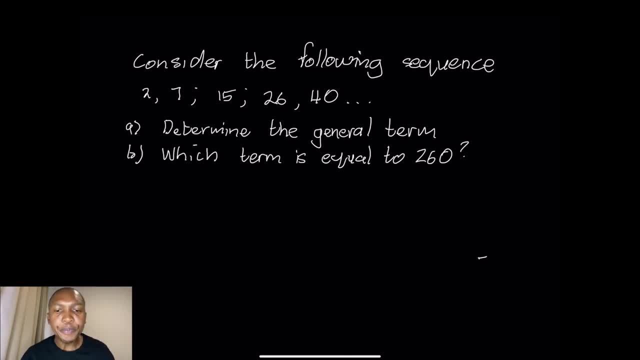 sequence: um, there, we've got that sequence there. they say: determine the general term first of all, and they say: which term is equal to 260? let's start with the first one. so is this a quadratic sequence? well, first of all, let's look at the um difference between the terms. 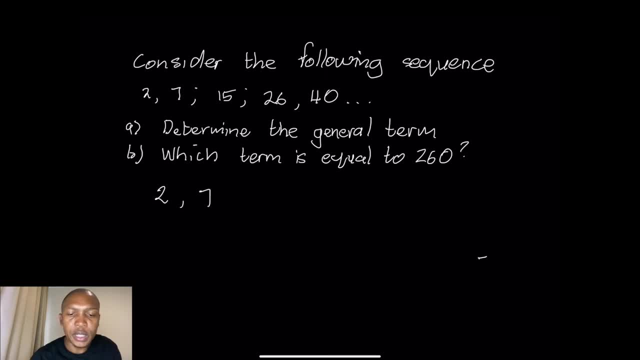 okay, uh, if you don't mind, i'm just going to um rewrite the terms. so i've got 2, 7, 15, 26 and 40. so if i take the first difference, okay, so i know, 7 minus 2, that would give me 5 um 15 minus 7. that would give me 8 um 26 minus 15. that would give me 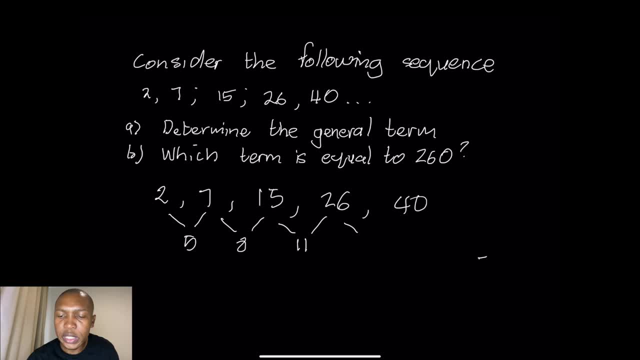 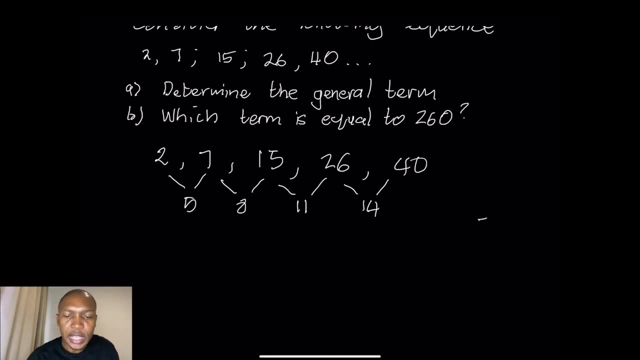 11 and 40 minus 26. that should give me 7. that would give me 8. um 26 minus 15, that would give me give me 14. okay, um, just verify and check if i'm correct and of course we can see that there's no. 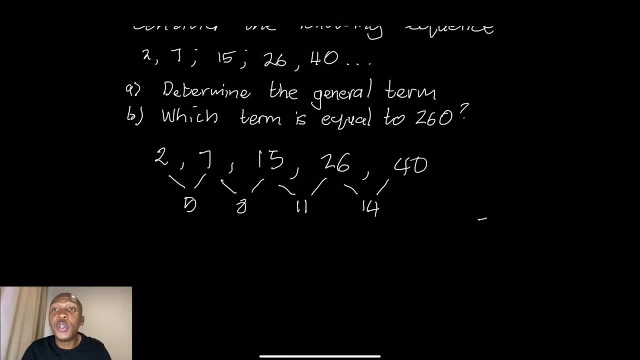 constant difference there. um, even if you tried the common ratio, you know, like we did for the geometric sequence, you'll see that it doesn't work. okay. so in this case, let's see if we take the second difference, so this would be 8 minus 5, that would give us uh, 3, um, if i took this, 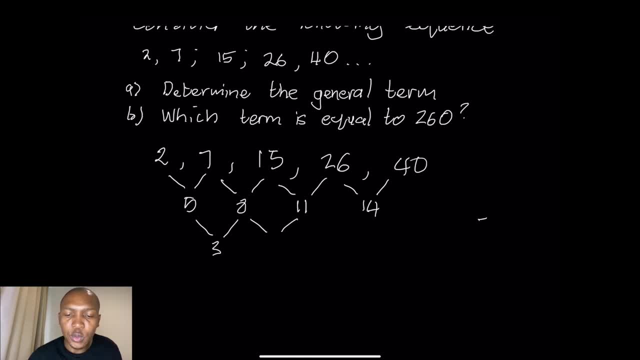 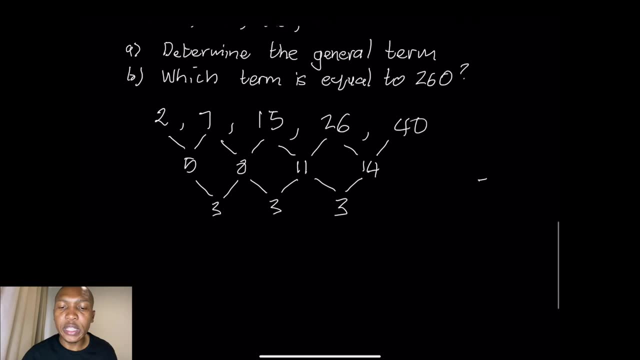 11 minus 8, um, that would also give me 3, and, of course, 14 minus 11 gives me 3. so now we've got a constant um common difference. uh, we've got a second difference, rather. so what i'm going to do now is let's go to our formula again. all right, so what did we say in order for us to find? we said: 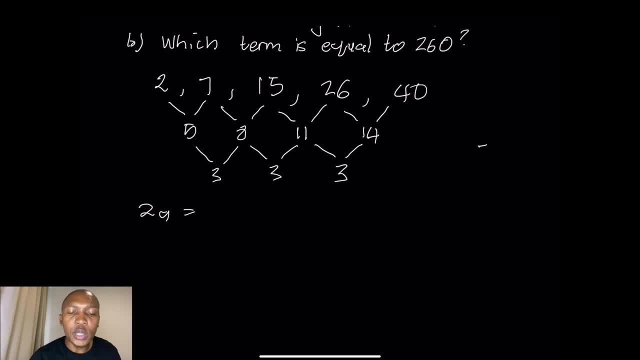 2a would be equal to the second difference. okay, so 2a is equals to 3 this time. so it means our a value would be 3 over 2. okay, and um for the b value. we did say that 3a plus b is equal to, in this case, the first term of the first difference. 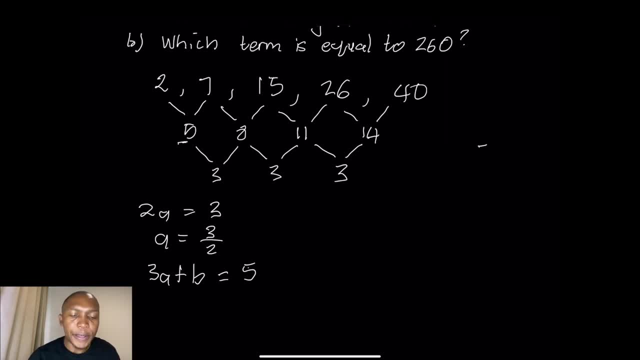 so in this case this would be equal to 5. okay, so we already know the value of a. so a is 3 over 2 plus b, this would be equal to 5. of course, we can simply just slip this into your calculator. um, so i get a b value of okay, let's check that quickly. um, so we'll say 5 minus, uh, 3 into 3 over 2. 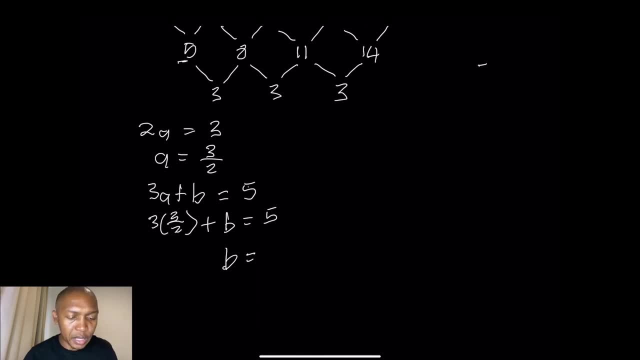 um, and that gives me a half. okay, right, um, am i correct? right, um? i get. yeah, so that's 5 minus uh 3 into 3 over 2. okay, and actually i made an error, i could see that. okay, so i get. i get 1 over 2. okay, so my b. 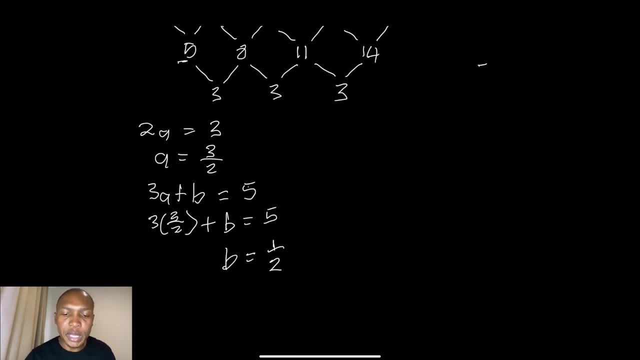 value is 1 over 2. so uh, and then i get a half. okay, so i get a half. okay, so i get a half. okay, so i get a half. in this case, that means that i can now find the c value. and remember, how did we find the c? we said: 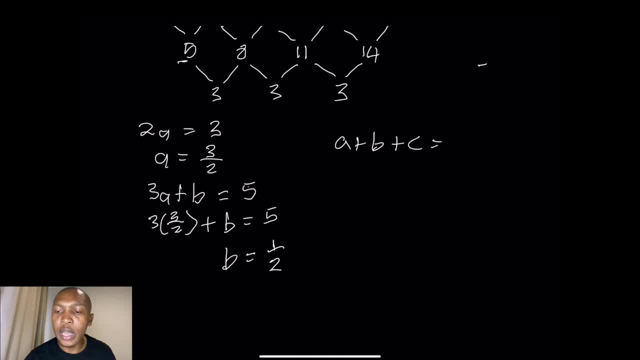 a plus b plus c is equal to the first term of our sequence, which is 2. so it means that i'm going to say: well, i've got my a value, which is 3 over 2, i've got my b value, which is 1 over 2 plus c, which. 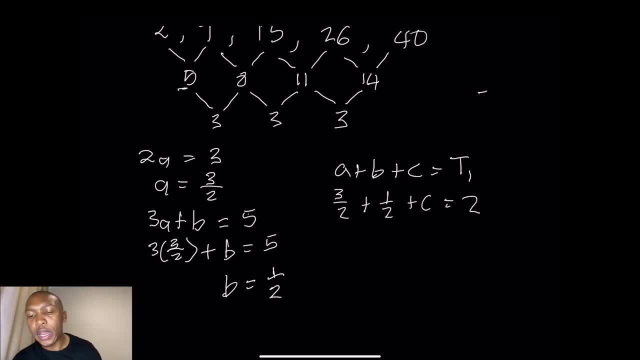 we are trying to find. this is equal to 2. now, if i take 3 over 2 plus 1 over 2, i get a half. okay, so 1 over 2. that gives me 2. um, so this is 2 plus c is equal to 2. so you can see how c will now be. 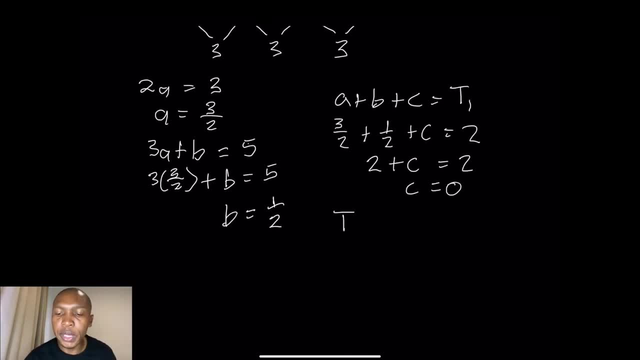 equal to 0. so it means that our general term will be: uh, tn is equal to the yeah, so that's 3 over 2 n squared, plus 1 over 2 n. okay, since c is 0. so this is the general term of this quadratic sequence. right now, going to the second question. 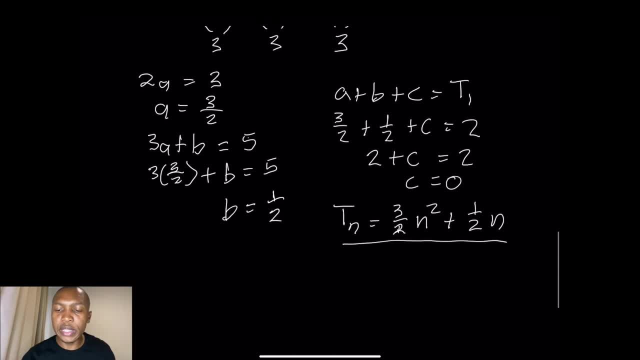 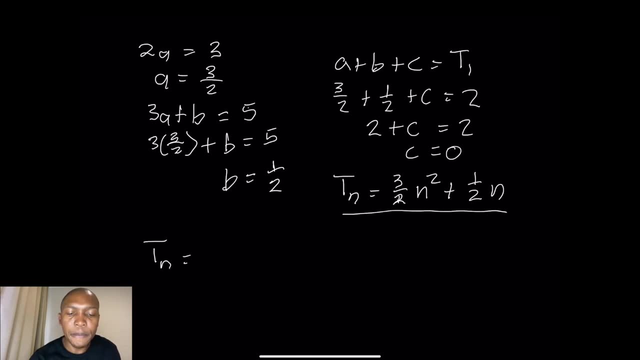 they said to us which term is equal to 260. so it means that now we're trying to find out. okay, so tn, um, so that's our b. so tn, that's 3 over 2 n squared plus 1 over 2 n, which term is equal. 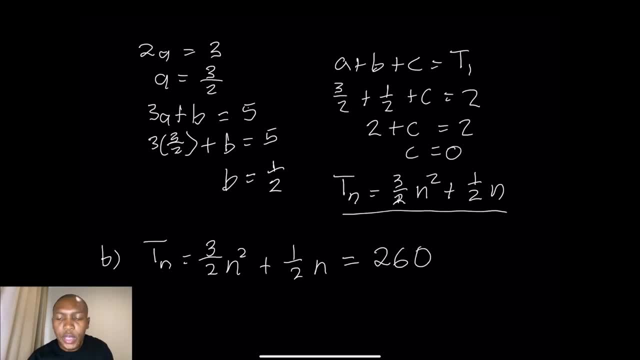 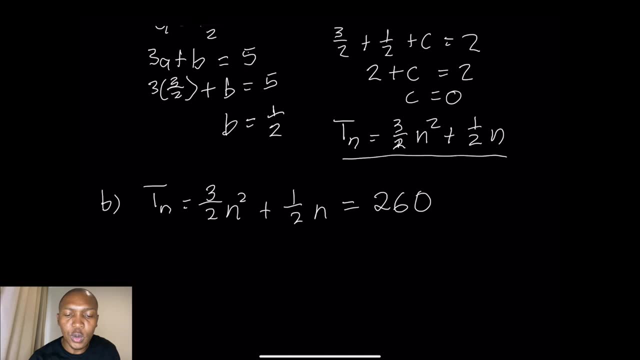 to 260. okay, so we're going to try and solve for the value of n there, okay? so, uh, we've got ourselves a quadratic equation, so let's try and solve that quickly. um, so we've got, uh, all right, so 3 over 2 n squared plus 1 over 2 n is equal to 260. now, to make this simpler for ourselves, let's: 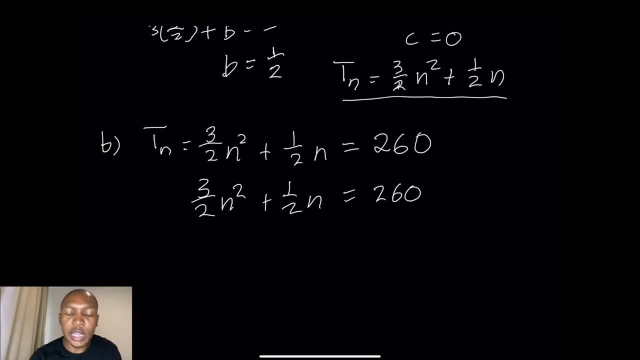 just multiply everything by 2 so that we just get rid of those fractions. so this is going to be: uh, if i multiply 3 over 2 by 2, that gives me 3 n squared plus n- okay, which is equal to um 520. that should be 520, okay. so let's try to solve. 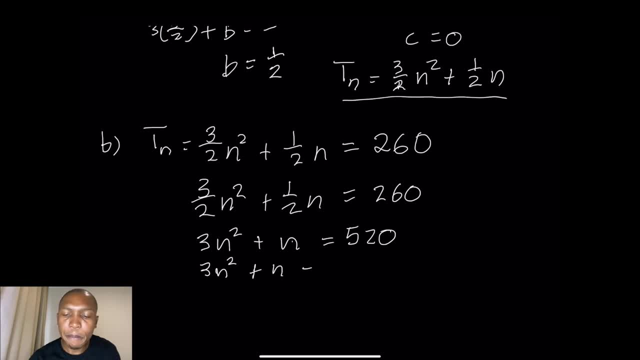 3 n squared plus n, minus 520, should be equal to 0, and, of course, what you can try to do is factor in the value of n. so let's try to do that. so let's try to do that. so let's try to do that. 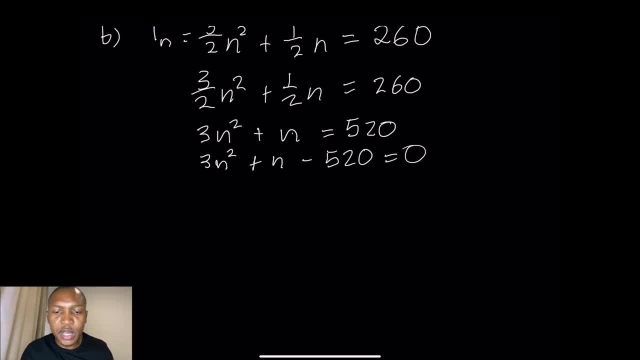 here and i am not going to try to do that. let's try and use the quadratic formula. in this case. i'm simply going to say this is: n is equal to: okay, and i hope that many of you probably know the quadratic formula, okay, so there's a way that i always try to do the quadratic. 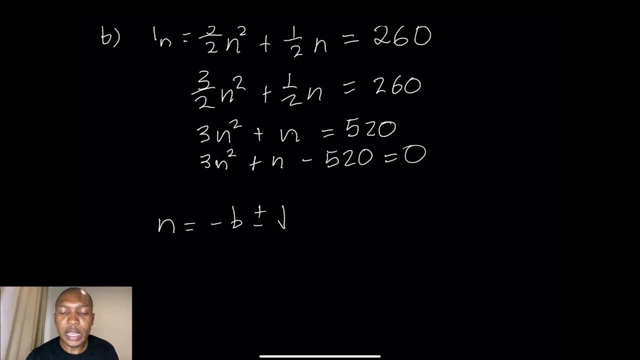 formula. that makes it easier for myself. so that's minus b plus minus. i know you'd say b squared minus 4ac, but let me leave that to you and i'm going to try to do the quadratic formula as delta. okay, we call that the discriminant right? sorry, i can't get that triangle correct. 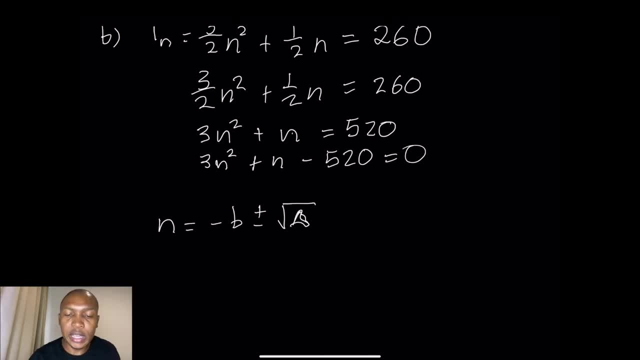 so i'm going to leave that as delta divided by 2a. you have to agree, this kind of looks neater, right? but you know that delta is equal to b squared minus 4ac. so what i do is i work out the value of delta on the side, and the reason i want to do that is that if delta is negative, 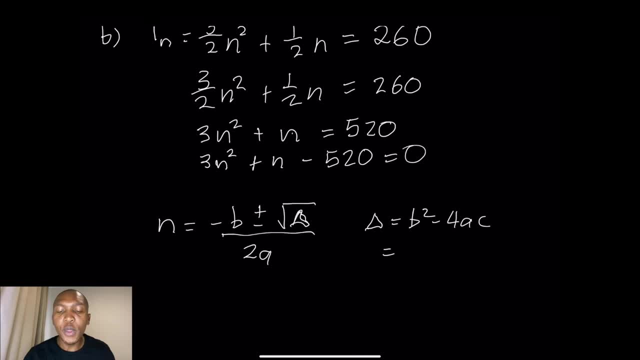 then it means that there's no solution to this thing. okay, without having to go through the entire formula to determine that. so what i do is i'm going to say: well, that's b squared, and my b value in that case is 1. so that's 1 squared minus 4 times. our a value is 3 and our c value is minus. 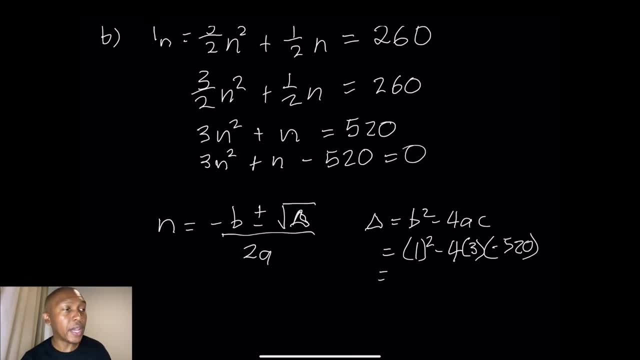 5- 20. okay, so let's find out quickly what the value of delta is. okay, so that would be 1. so remember negative times a negative here, so it's negative times. negative 4 times 3, which is 12 minus 12 negative: 12 times a negative: 5- 20. so i'm going. 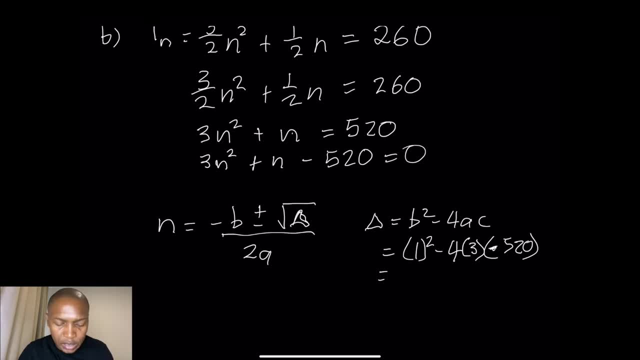 to have so 4 times, 3 times 5, 20. okay, so i get- okay, that's obviously that would make that positive plus 1. okay, so i've got 6, 2, 4, 1, so we can take that value. um, it's a positive value, so it means that. 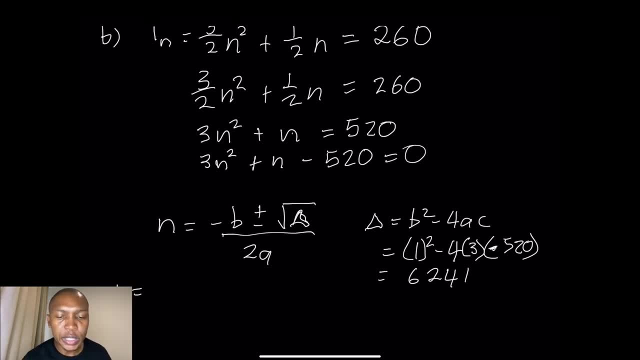 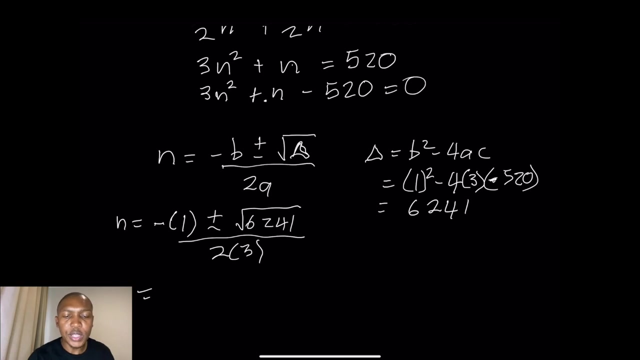 of course i am going to get real solutions in that case. so let's substitute: so minus b, so we've got minus. remember, b value is 1 here. so that's minus 1, plus or minus the square root of that number, 6, 2, 4, 1, divided by 2 times our a value is 3. okay, and finally, let's get an answer to that, of course. 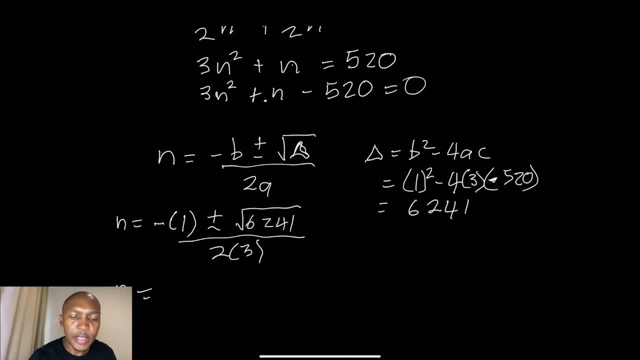 the first one would be a negative. so n is minus 1 minus. what's the square root of that whole number? okay for answer: it's 79. so the square root of 6, 2, 4, 1 is 79 minus. what's the square root of that whole number? okay for answer: it's 79. so the square root of 6, 2, 4, 1 is 79. 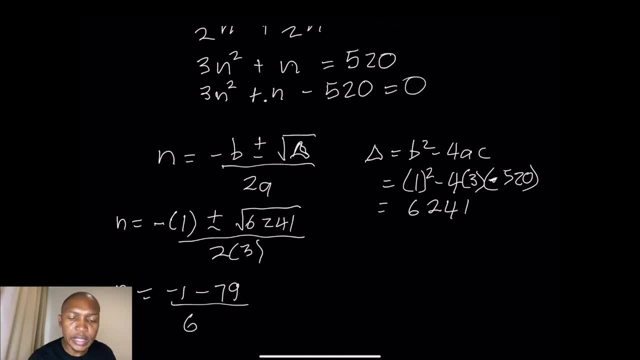 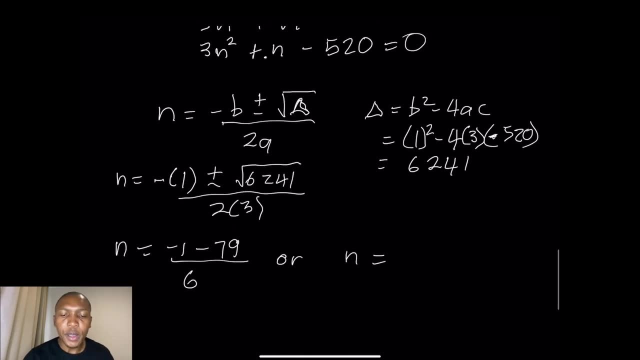 minus 79 over 6, and of course you can see how that is not going to be applicable. okay, so that's going to be minus 1 plus 79 divided by 6. okay, so i've got two solutions here: 76, um, so that's. 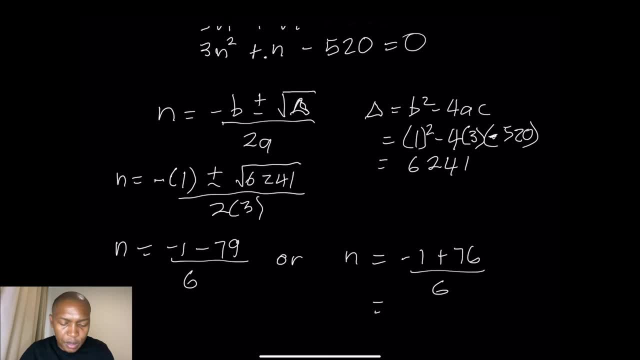 divided by 6. okay, um, i think i just did something wrong here. i wrote 76 instead of 79. okay, all right. okay, so that's 79. okay, so i've got 78 divided by 6 and i get a value of 13. so my 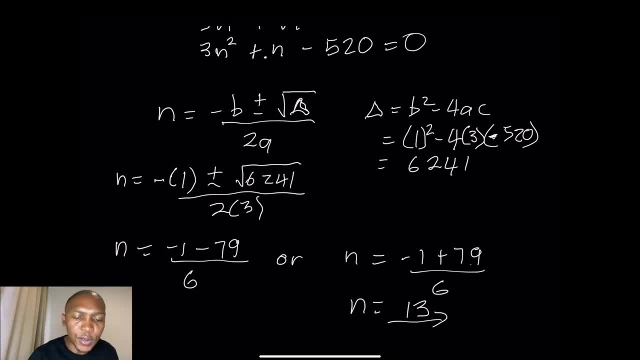 solution? my answer is that i'm going to get a value of 13 and i'm going to get a value of 13 and, of course, over this side, you've got 80 minus 80 divided by 6, um, in which case you get minus 13.33. uh, but this one is definitely not applicable. why? because we cannot have 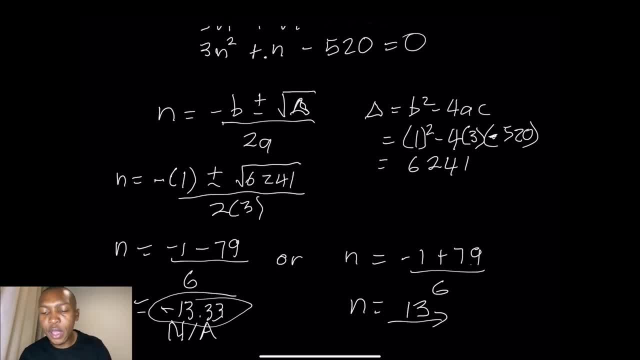 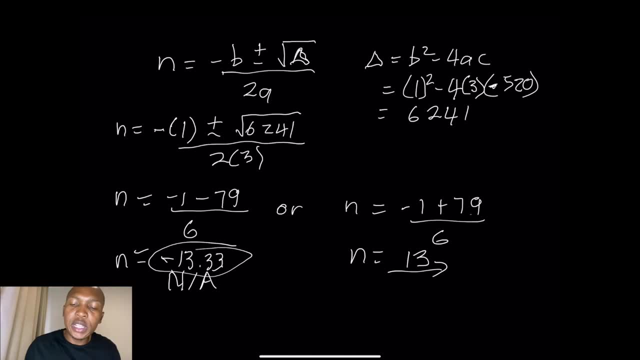 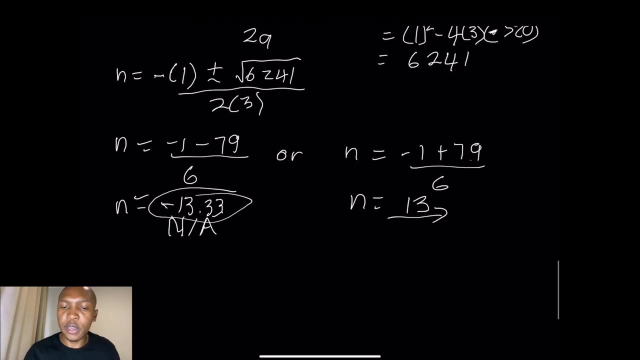 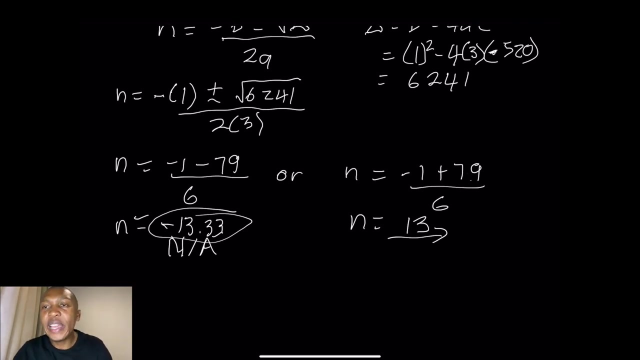 a negative term. okay, remember, we are increasing, going that way, um, in that case. so our final answer: it means that the 13th term of this quadratic sequence is equal to that 520 value that was given. all right, and this is where i would love to leave it, ladies and gents, i think it's been a fruitful one. thank you so much.